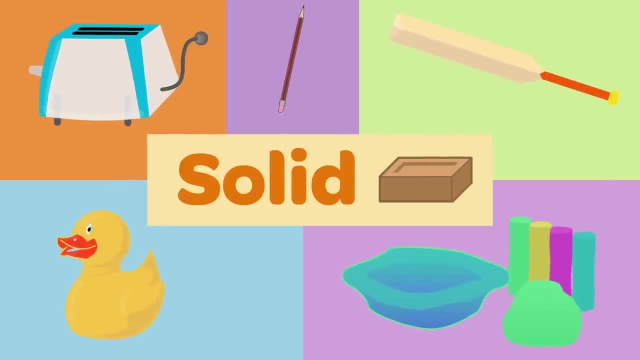 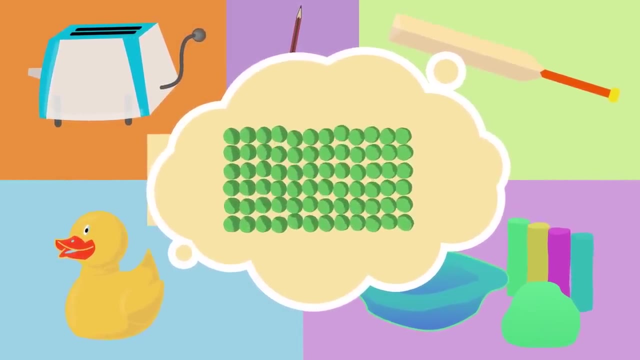 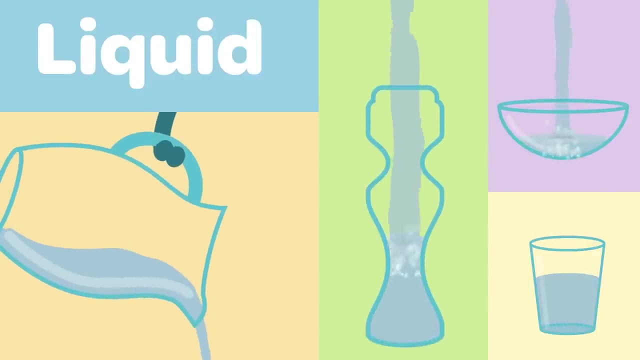 rubber toy or a piece of clay. Solid means that the atoms are packed in really close together so they can't move, which means the object holds its shape. A liquid, on the other hand, will always change its shape. It changes shape to fit the shape of the container it's put in. A liquid can 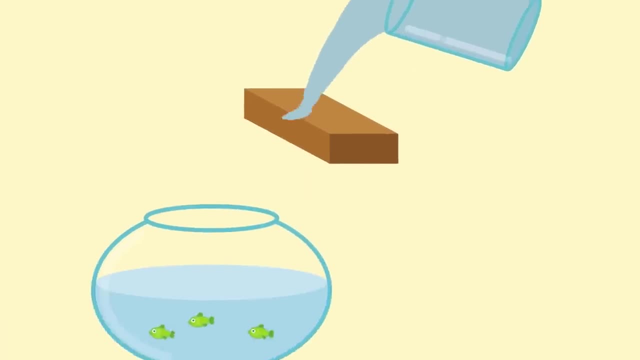 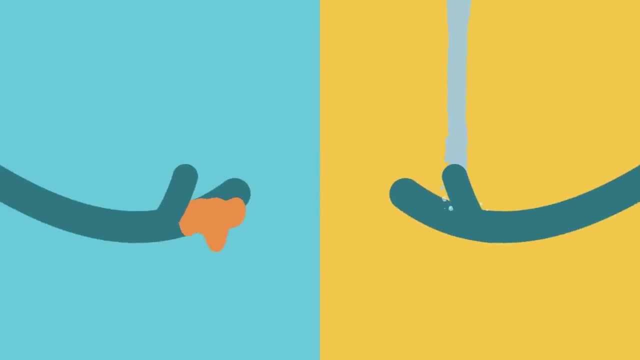 flow, which means it can be poured. So if you pour water into a fishbowl, it moves to become the shape of the fishbowl. There are many ways to use the liquid. For example, you can pour it into. liquids are sometimes thick like honey or thin like water, but no matter what, they'll always flow. 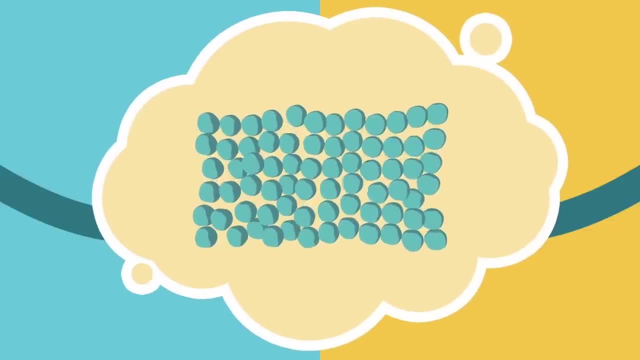 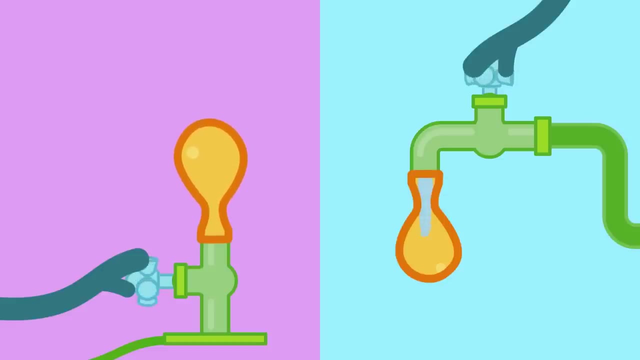 atoms in a liquid can move around, but they'll stay together. a gas, like a liquid, takes the shape of the container it's in but will also spread out to fill the container. when a balloon fills with water, the water fills up the bottom first, but when you fill it with a gas, the gas 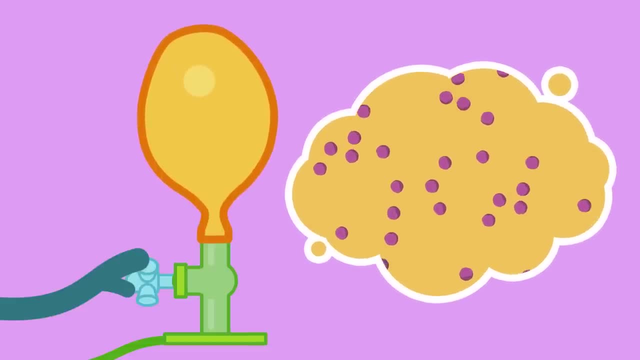 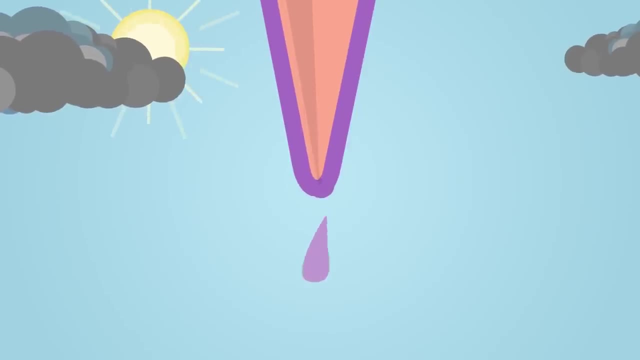 fills the whole balloon. sometimes matter can change states, usually by changing its temperature. if you heat ice cream, it will melt and turn to a liquid. if you make the ice cream cool again, it will then turn back to a solid. water is unique because it's the only thing on earth that naturally 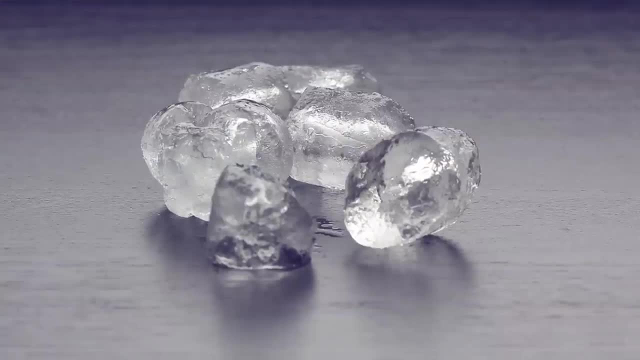 occurs in all three states as a solid, as a liquid and as a gas, and it's the only thing that naturally occurs in all three states as a solid, as a liquid and as a gas. and it's the only thing that naturally occurs in all three states as a liquid and as a gas, and it can change states quite easily. water in. 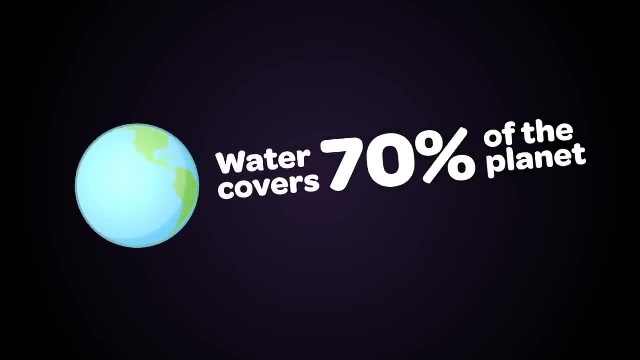 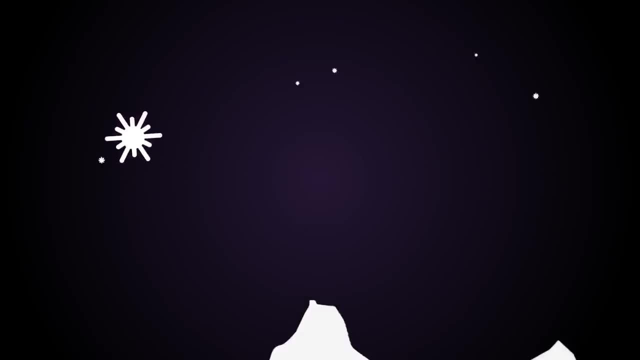 can change states quite easily. water in its most common form as a liquid covers about 70% of the. its most common form as a liquid covers about 70% of the planet. it also has no taste, smell or color planet. it also has no taste, smell or color. water constantly changes states in nature in very cold. 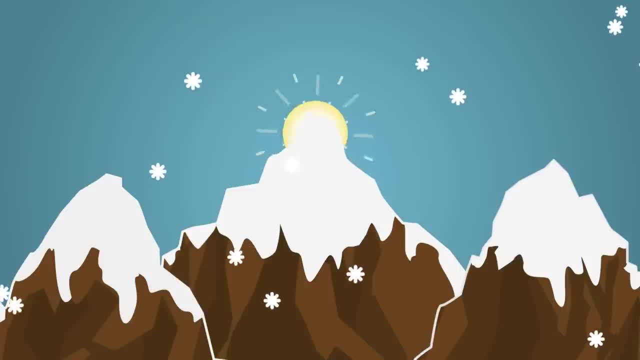 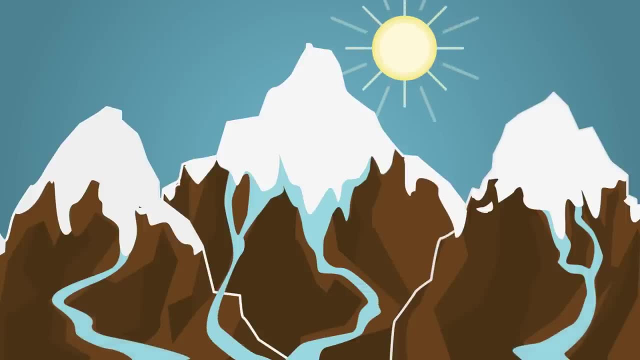 water constantly changes states in nature. in very cold places like the mountains, the water freezes. places like the mountains, the water freezes into ice and snow. the Sun then warms the frozen water into ice and snow. the Sun then warms the frozen water, causing it to melt to liquid water as the